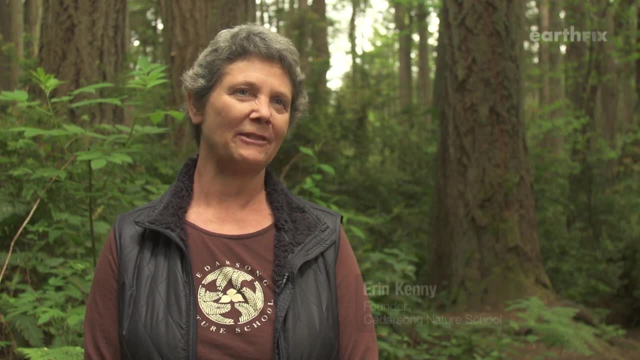 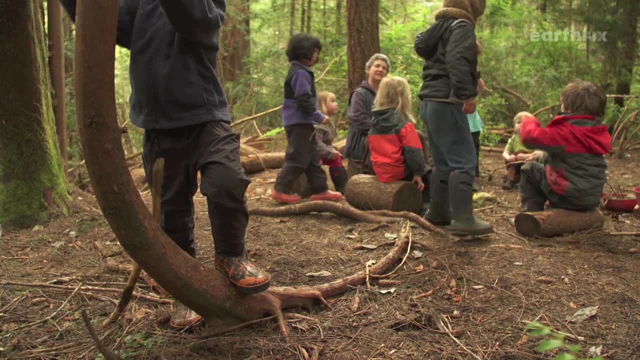 They're just doing it outdoors and naturally at their own pace. Cedarsong opened in 2006 on Vashon Island, a short ferry ride from Seattle. Does anybody have a story they'd like to tell? It was the first forest kindergarten in the United States. 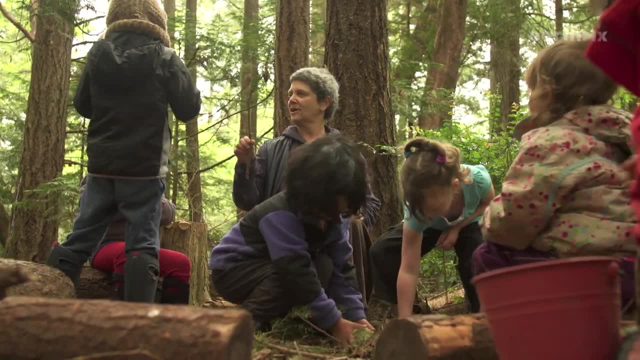 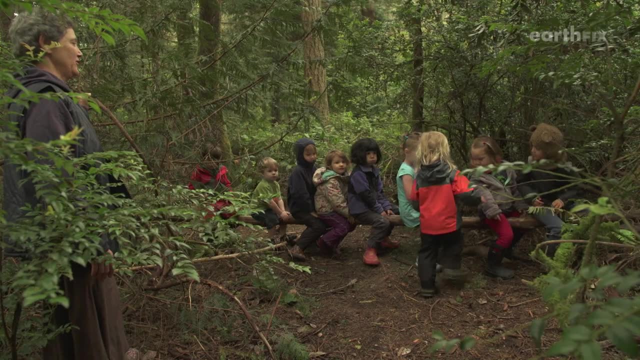 Kenny built the school in response to the alarming trend she was seeing American children spending less time playing outside. Elizabeth, you want to get on? They're stopping the bus. And when kids stay indoors, Kenny says their connection to the natural world withers. 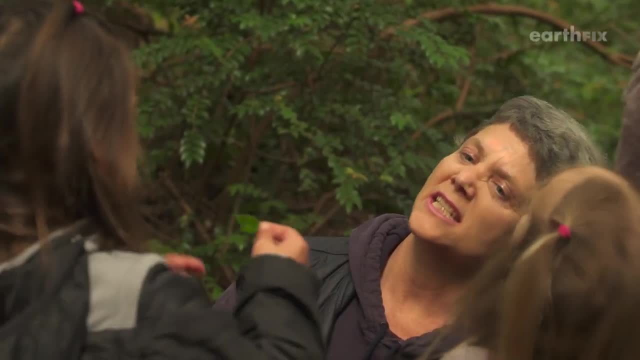 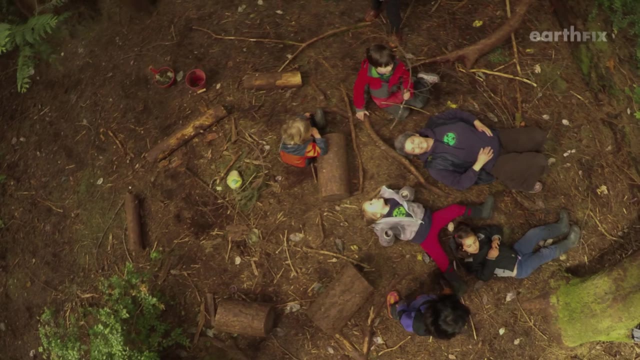 Way up there, I see it. Do you see way up there? Yeah, Does anybody want to lie on the ground? Learning outdoors was one of the best ways to create a positive and intimate bond with the natural world, But what happens when the weather turns cold and rainy? 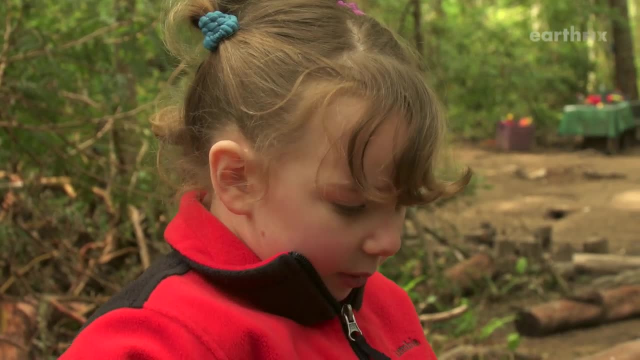 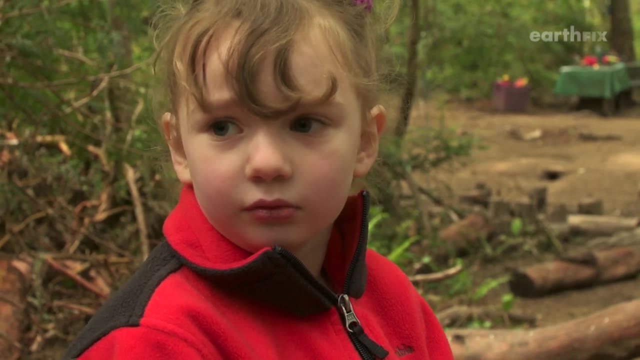 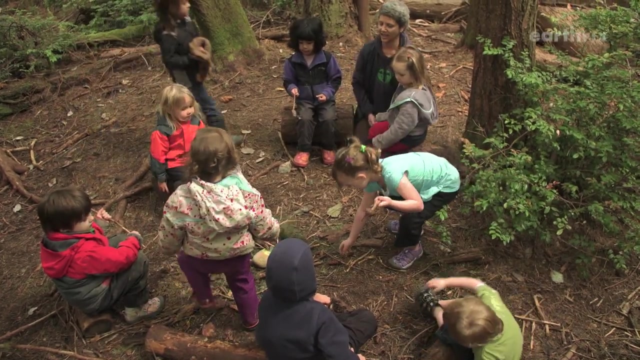 Well, we put on a coat if it rains and we put on a face if we get cold. My lips are turning blue. right, The children have no problem with the weather, no matter what the weather is. Once children are appropriately dressed, they can spend many hours in nature with no cares. 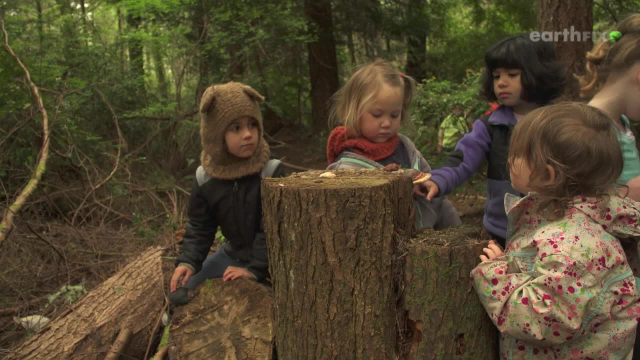 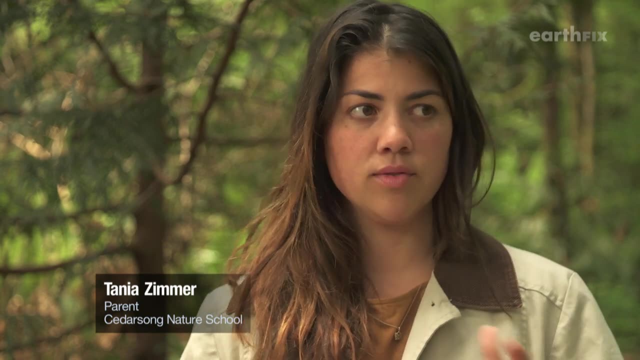 Cedarsong parent Tanya Zimmer agrees I've never really had an issue with them with the weather. They've never complained about it once. I think it builds a certain amount of resilience and grit. Zimmer says her two-year-old daughter, Tanya Zimmer, has a lot to learn. 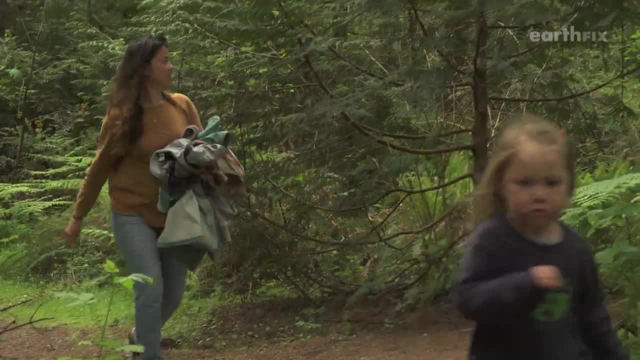 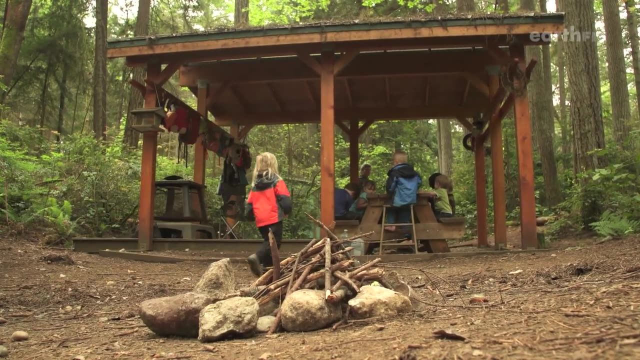 Her two daughters love going to school outside. There hasn't been a day where they have not wanted to come to the school or they've left in a bad mood. Now, a decade after Cedarsong started, the outdoor school idea is growing. 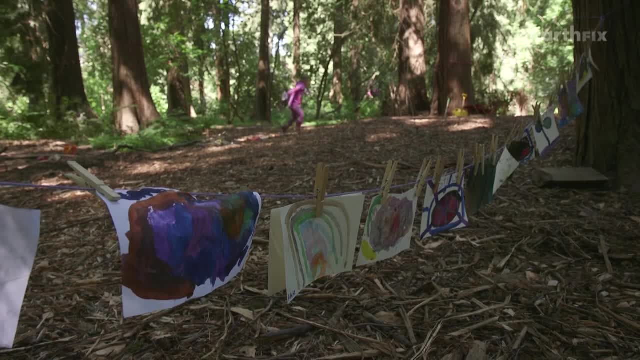 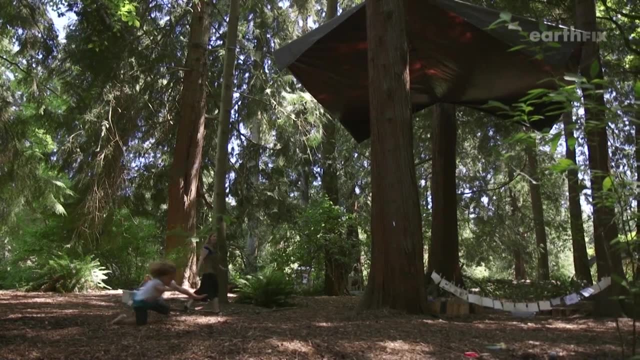 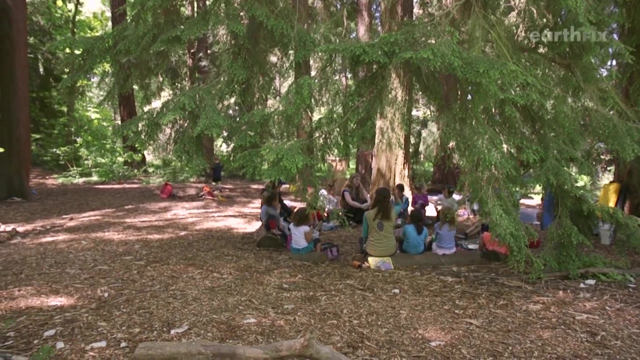 Similar schools have sprouted across the nation. In the greater Seattle metropolitan area alone, there are now more than two dozen outdoor schools. One is the Fiddleheads Forest School, nestled among the towering cedar trees of the University of Michigan. Another is the University of Washington Botanic Gardens. 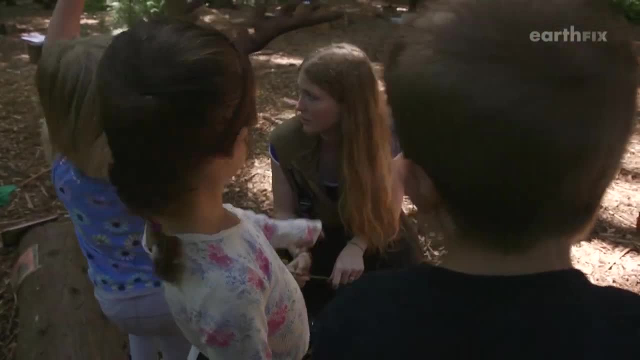 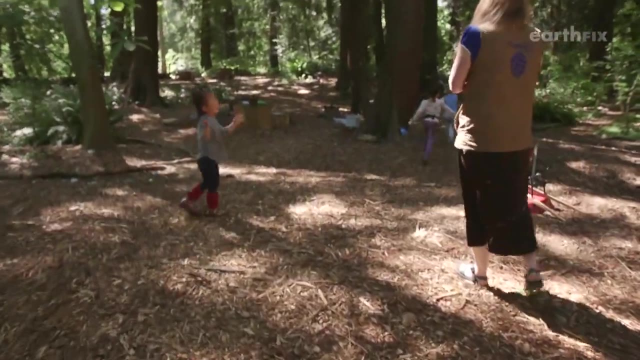 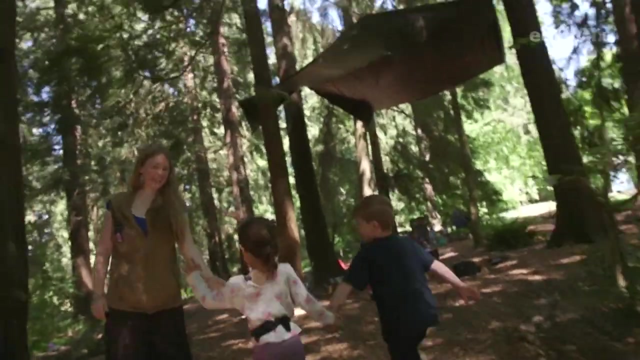 Does anyone else want to run around the classroom before lunch? Mina, you want to go too, Aria you want to go too. Okay, let's get out some of our energy. Teacher Joanna Wright says she noticed an inherent benefit to outdoor preschool.